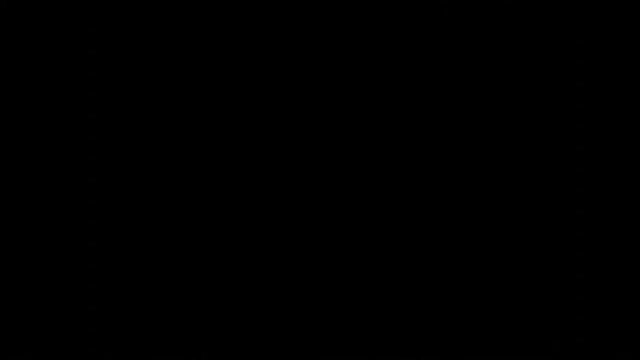 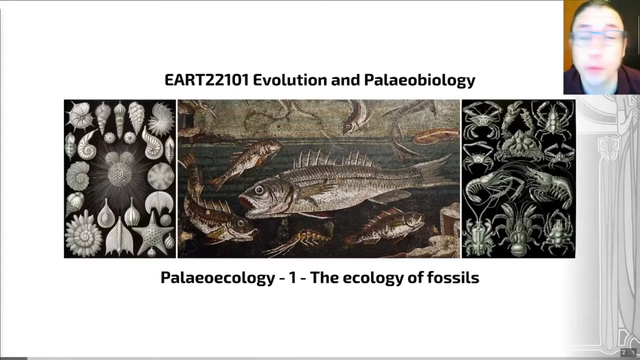 Hi there and welcome to the first video of content on paleoecology in which we're going to be looking at the ecology of fossils. So I noticed when I was recording the last video that I was actually maxing out the volume on my inputs, so I apologize if that was the case and 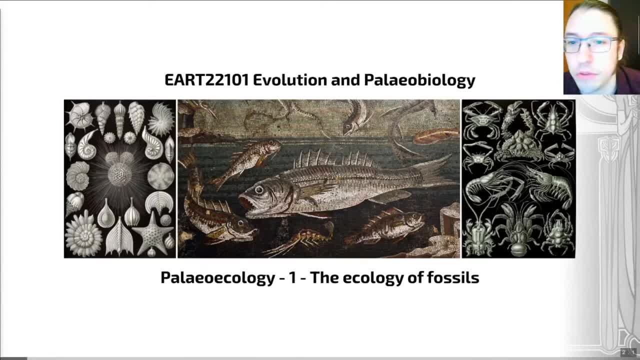 now I seem slightly quieter. Nevertheless, I hope that the audio is okay. So in this particular video, what we're going to be looking at is what ecology and then what paleoecology actually is. So we'll then be moving on to what we can say about individual fossil species and how we can. 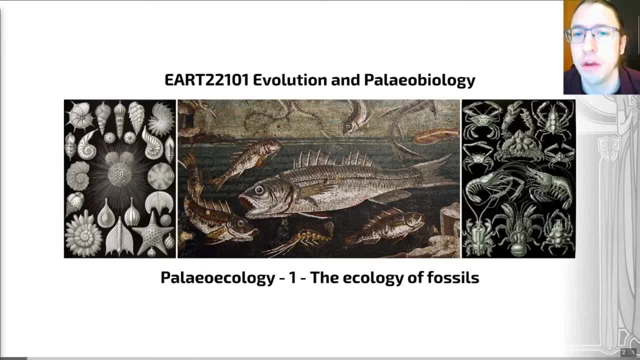 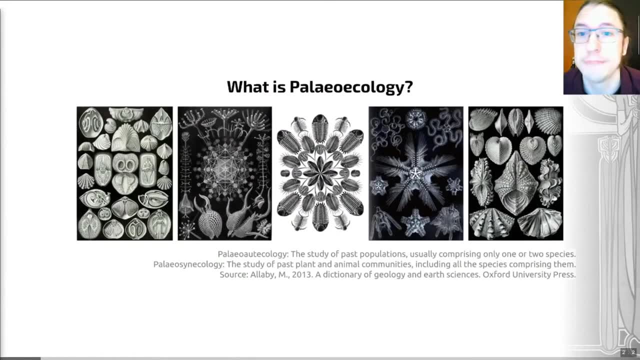 tell this and then we'll have a quick look at some examples allowing us to understand the ecology of extinct groups of animals. I hope that'll be pretty cool. I'm looking forward to it, But I I'm a strong believer that um in defining terms, when we start stuff to make sure that we're all 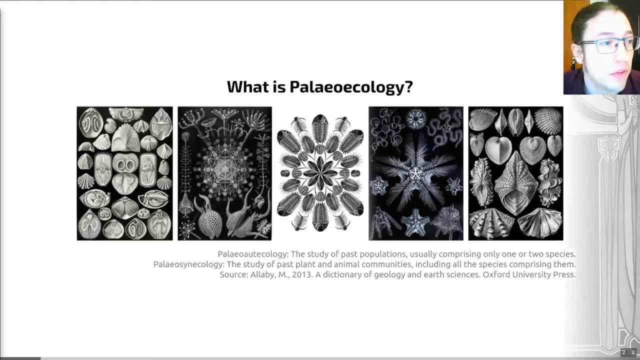 on the same page. So here you can see on this slide some examples of a range of groups of fossils, or groups of animals, I should say, with a very rich fossil record. How can we use these to understand ecology in the earth's past? This is a key to defining the question: what is paleoecology? 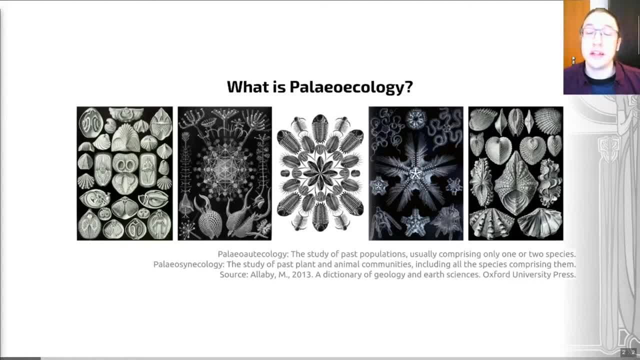 So, if we want to define our terms, the definition of ecology is the branch of biology that deals with the relations of organisms to one another and to their physical surroundings. That is a definition of ecology for you, thanks to the Oxford English Dictionary. So it's basically looking at interactions, as much as it is the 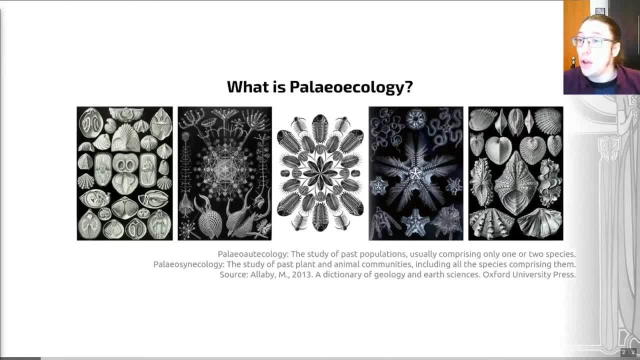 actual biology themselves. Paleoecology is just the application of these principles and these questions to the past. Perhaps a useful way to look at this and make it seem a bit less intimidating, because it's a very broad field- is to split it roughly into two different camps. 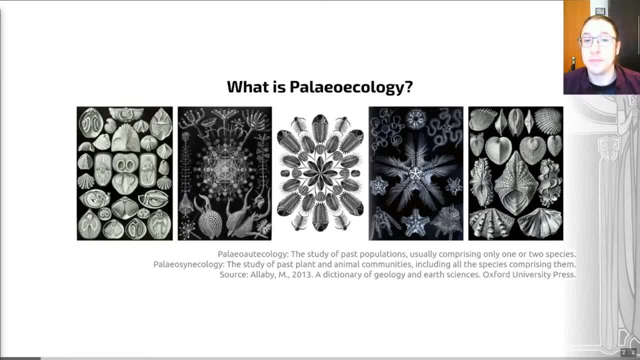 We can look at the ecology of extinct species, so we can look at the role they play in their ecosystem, their mode of life and their feeding and their breeding habits. This is a thing called paleo-auto-ecology. I've placed a definition of it on the slide for you. 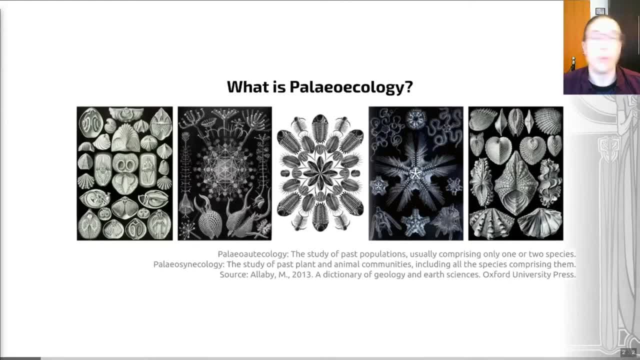 here the study of past populations usually comprising only one or two species. so in short, this is kind of zoomed in paleoecology. but we can also use geological and fossil evidence to reconstruct past biotas as a whole. we can understand, above populations, whole communities. 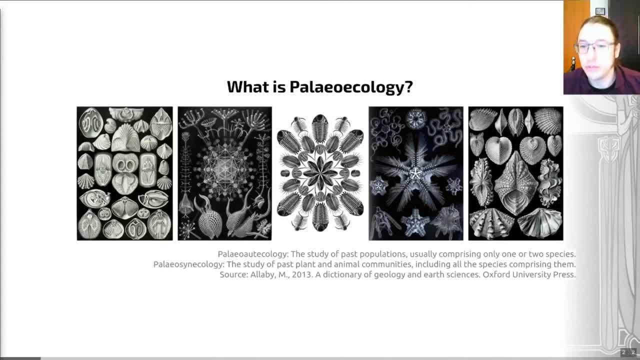 landscapes, environments and ecosystems. this we could call, if we wanted to, paleocynicology: studying these complex interactions between populations of species, within communities of organisms and within ecosystems as a whole. i've also put a definition of this on the slide for you, and that says paleocynicology is the study of past communities, including all the species. 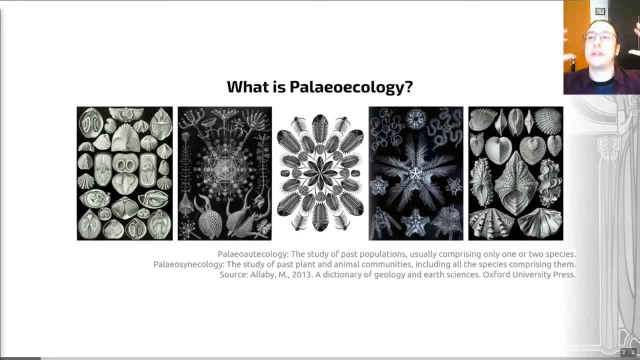 comprising them. so basically, this is the zoomed out bit of paleoecology. that's a fairly arbitrary and semantic, i think, division, but nevertheless it's one that helps us divide this up slightly into bite-sized chunks. i think that's necessary because there are a wide 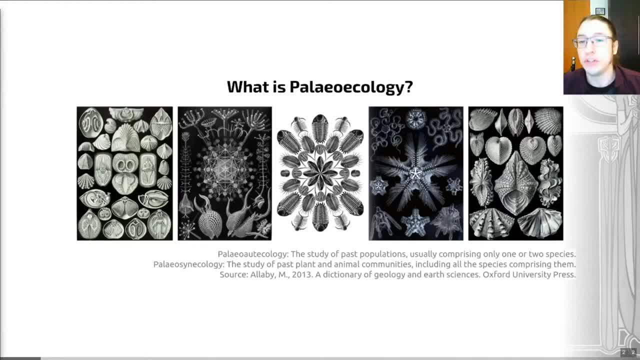 number of ways in which you can do paleoecology. it's actually a really interdisciplinary field, drawing on lots of different strands of different sciences, so i hope that's a useful definition and useful division of this science for you, and i wanted to highlight that paleoecology 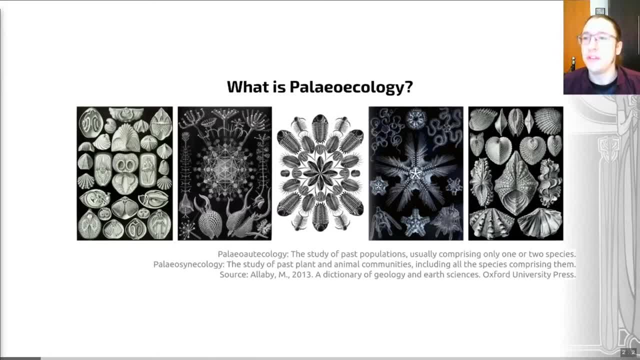 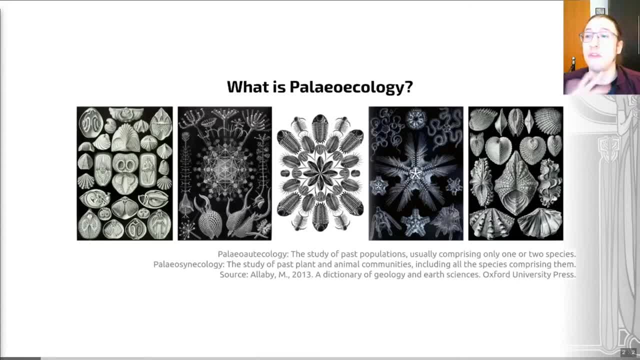 and less evidence. as we get older and older, we have fewer and fewer rocks which will be holding fewer fossil species as we go deep into the geological past, and that can limit what we can say about past ecosystems, but also because the further you go back from today, the increasingly 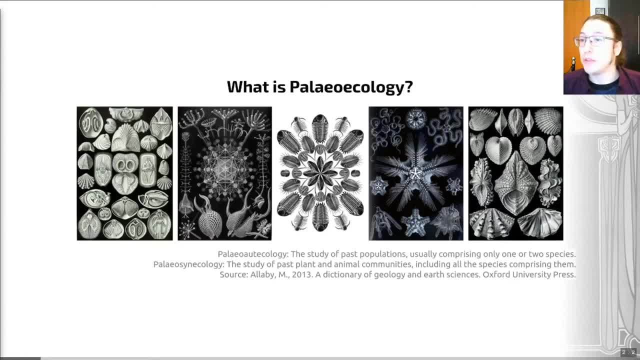 dissimilar those um ecosystems were- i'm sorry, that was an incredibly poor choice of words- increasingly dissimilar. basically, the further you go back in time, the more different ecosystems become to today, and what this means is that, as we go deeper into the past, uniformitarianism. 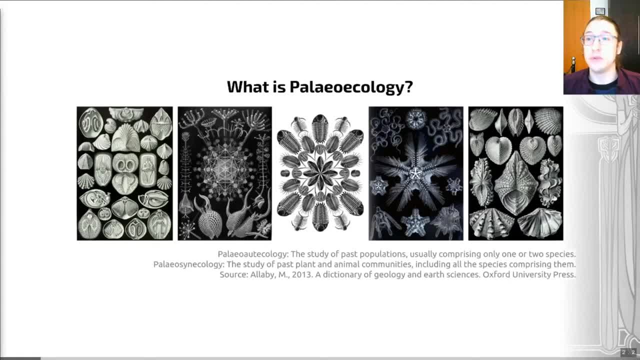 the idea that things happened in the past as they do today becomes increasingly difficult to apply because the animal communities that were around at those times have a very different makeup to those that are alive today, so i hope that clarifies my poor choice of words there for you. 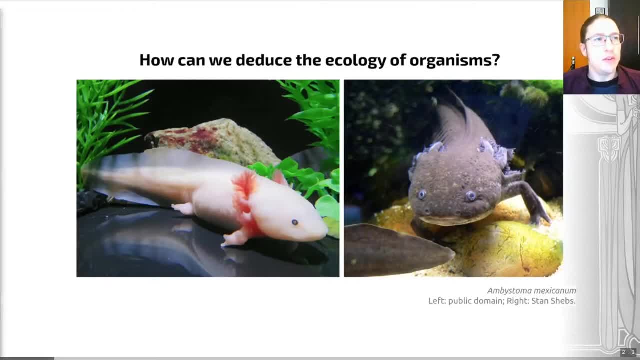 so how can we deduce the ecology of organisms and indeed individual species? so often when i'm i'm going to use these two interchangeably because we have one or two fossil exemplars of all of these ancient species. well, paleo, autoecology, the branch of ecology that deals with this particular 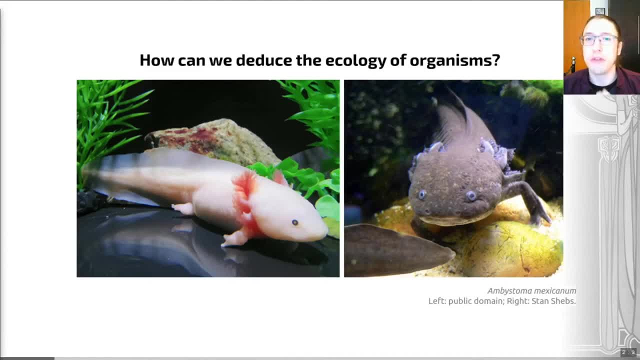 question broadly looks at, when we're looking at the fossil record, the mode of life of fossil species, their life traits, including food and food sources: food and water and that's a very important- breeding and feeding, for example. so this is kind of like the bread and butter of paleo autoecology. 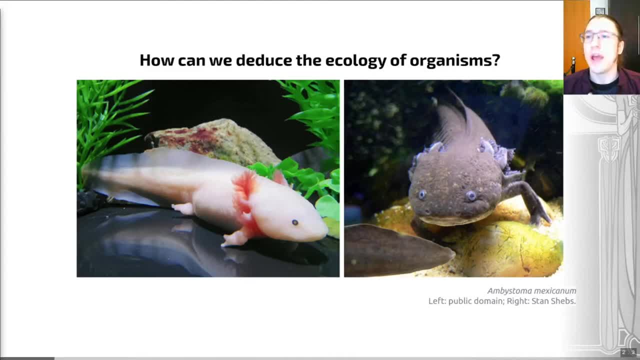 what we can actually say about individuals, but also how they fitted into the ecosystem of which they are a part. this is primarily achieved through functional morphology. this is the field in which we deduce the function of the part of an animal from its morphology. so the clue is in its name. 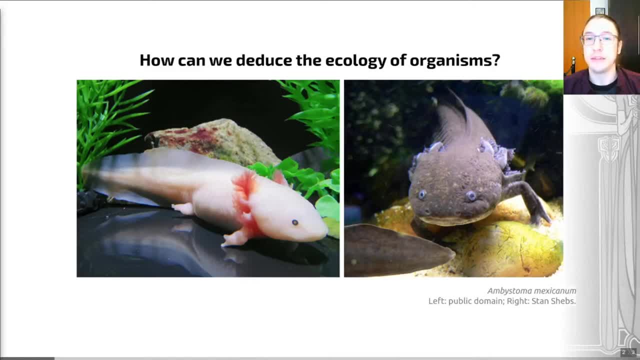 it's using the anatomy of extinct creatures to say things about their mode of life, so that's essentially how their morphological form is related to their function. we can combine lots of pointers from different parts of the anatomy of these of fossil creatures to get a clearer idea of the mode of life that they- um, they had and therefore, 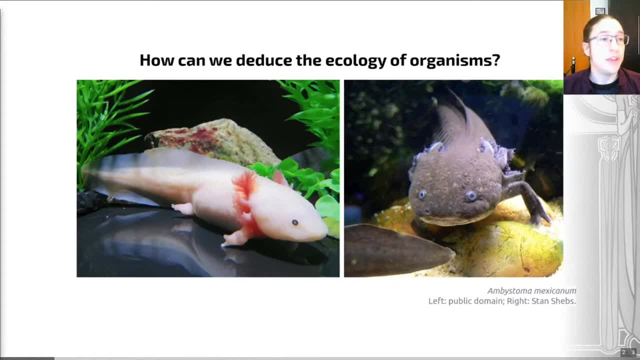 how they fitted into their ecosystems. my living example that's shown here is the axolotl which is shown on this slide. so this is the axolotl which is shown on this slide. is the axolotl which is shown on this slide. 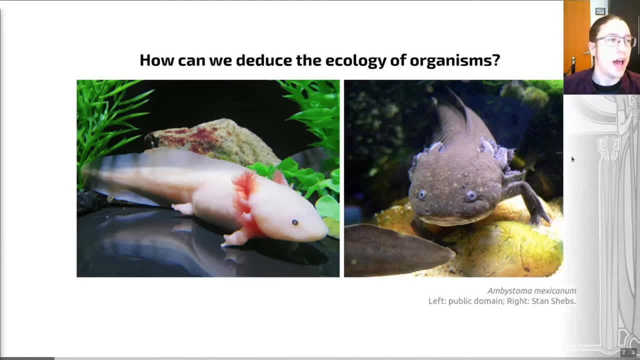 in its juvenile form on the left-hand side and in its adult form on the right-hand side. So this is an amphibious creature that is found in a few different environments. I often associate them with caves. I'm not sure exactly how accurate that is. 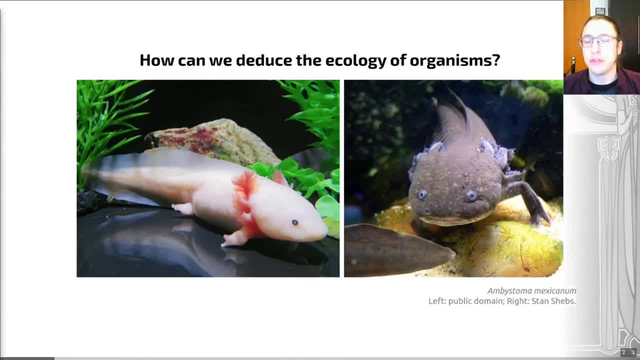 But we can tell just by looking at this fossil, this fossil, these aren't fossils. I've got no idea what the fossil record is like for these animals. We can tell by looking at just the shape, the morphology of these creatures in this slide. 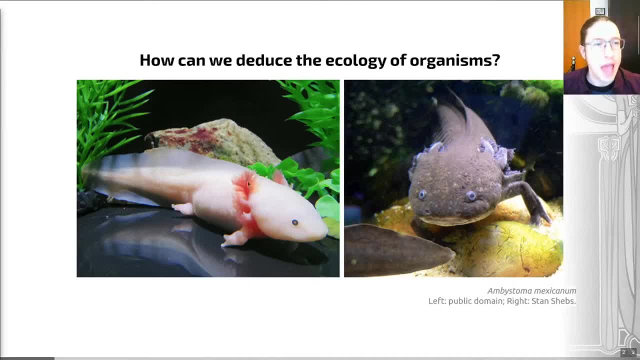 that they live in water. They have these beautiful external gills in both the juvenile and in the adult form, And that tells us that they are breathing underwater. They have a flattened tail for propulsion. This is far better for swimming than, say, a conical tail. 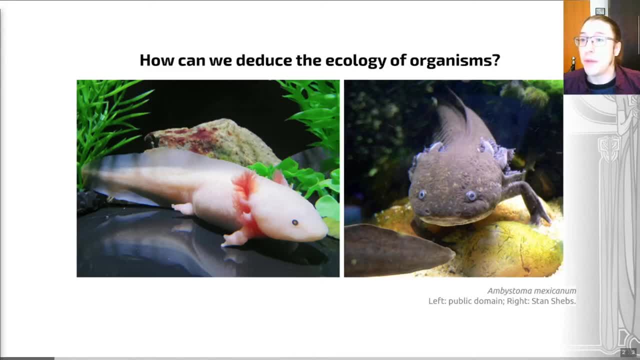 And so by just looking at that anatomy, we can say something about their mode of life. I wanted to highlight, since we're here talking about axolotls, that they're unusual among amphibians because the adults shown here on the right remain aquatic and gilled. 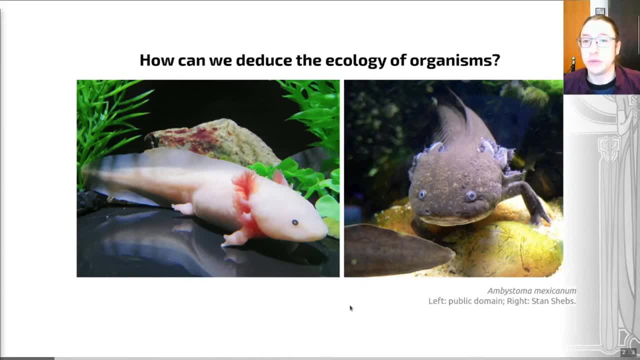 Mostly amphibian adults, move out of water And indeed these creatures are weird generally because they often don't even undergo metamorphosis, because their juveniles can breed So often. these creatures will stay in their juvenile form for their entire life And breed as juveniles rather than metamorphosing. 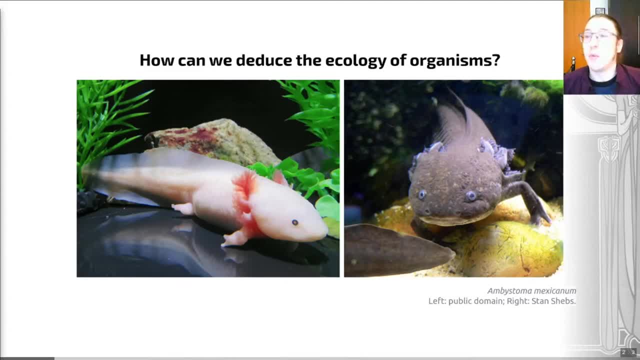 into this adult form. Also, top tip, they have a weird swallow reflex And that means that if you ever keep them as pets, you can keep these in fish tanks. If you feed them with food with lots of air, they then start floating. 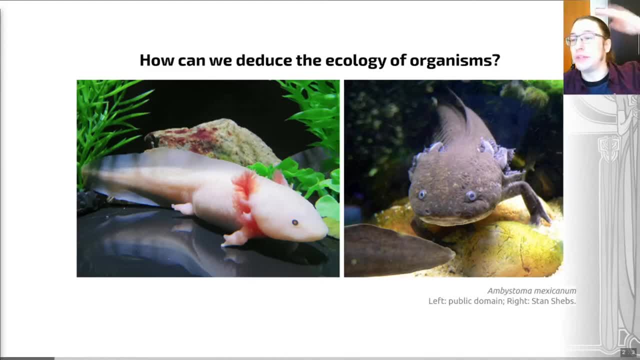 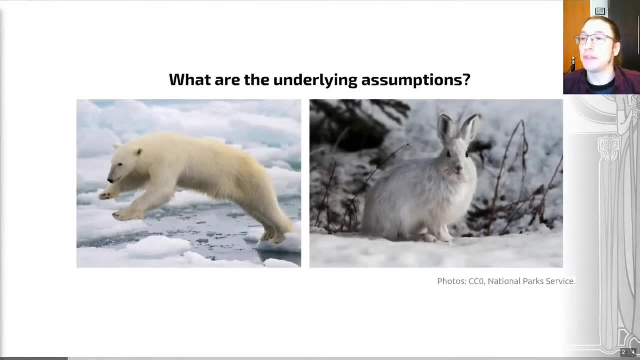 so they can't get rid of the air in their food And they float in the water column until they fart, where they sink again, which I think is really super cute. So they're really nice creatures in general, But they're my example of functional morphology. 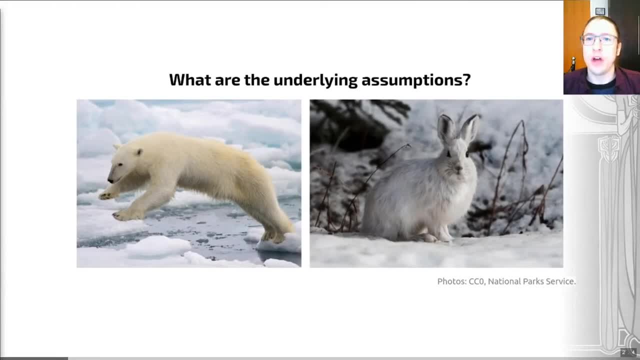 All of that works And you can see that they're very flexible because organisms are adapted to and primarily reside in a particular environment. How flexible they are obviously differs across the tree of life and within different groups, So you have things that are generalists. 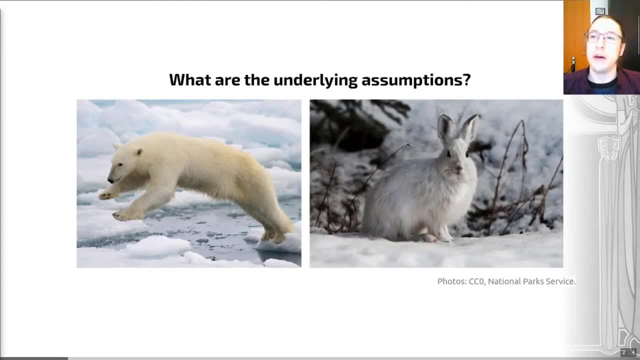 and these specialize less to their particular environment than specialists do. So generalists versus specialists. We can dig down deeper into that way And say that organisms are not only adapted to their particular environment in the majority of cases, but they're also adapted to a particular lifestyle. 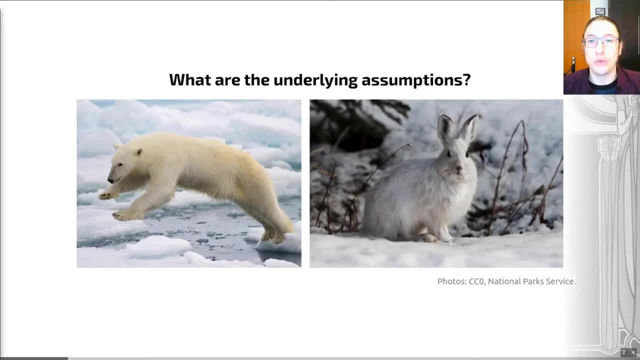 within an environment. In the example shown on this slide, both of these creatures- the polar bear on the left and the- I forget that's not an Arctic hare. Maybe it is an Arctic hare, The rabbit type creature on the right hand side. 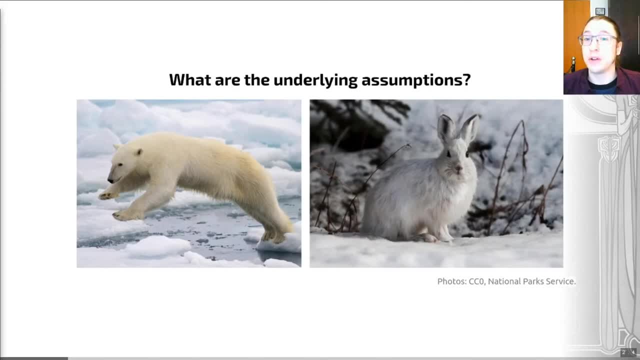 are both adapted to a lifestyle in Arctic environments, But they play a very different role in the ecosystem, with the polar bear being an apex predator and probably eating our creature on the right there, And this reflects the fact that organisms all interact with each other directly or indirectly. 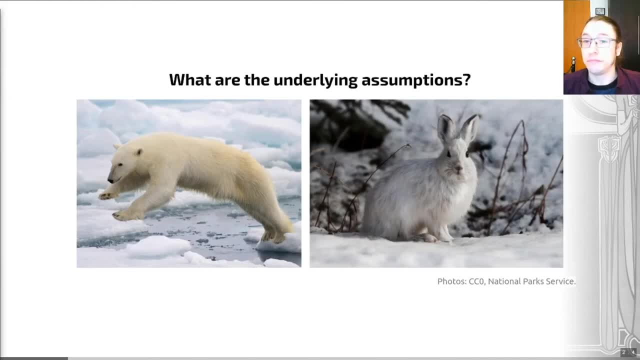 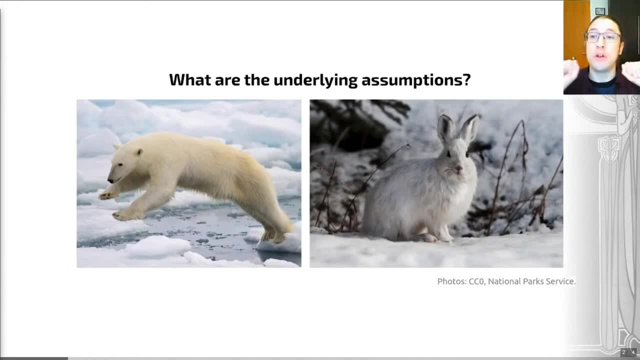 a species and its environment, but also the relationships between the different species within an ecosystem. so, within a particular environment, Uniformitarianism does apply. So this is the idea that we can use processes that occur today and relationships that we see in living organisms to infer things. 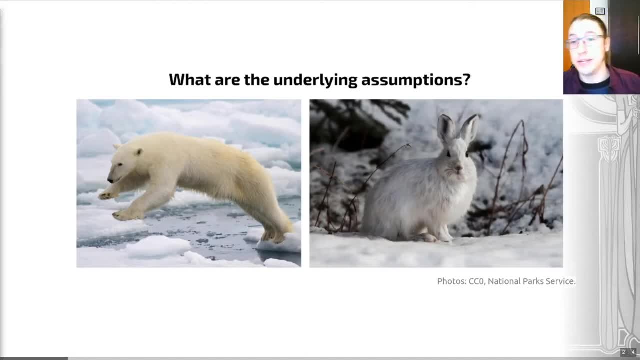 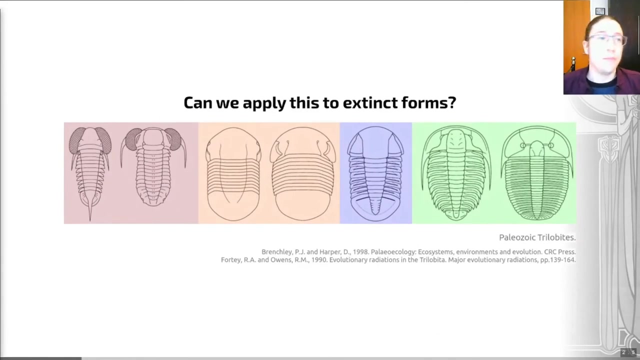 for fossil ecological communities. So we can make inferences about ancient organisms and environments based on analogies with organisms that are living today. Okay, so let's have a quick example of how we apply this to extinct forms. So here's an example of an extinct group. These are the trilobites, You know the 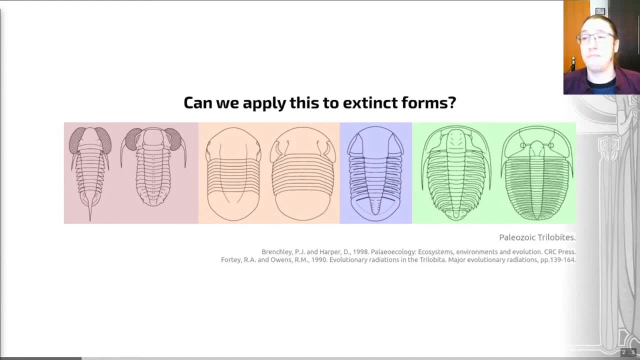 trilobites. very well, by now I'm led to believe you created a pretty awesome phylogeny for the group in your cladistics, practical just a couple of weeks ago, And this group develops over geological time a range of different morphologies and atomies that are associated with different modes of life. 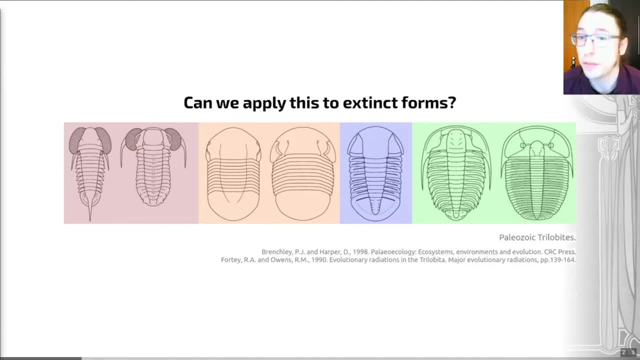 So the trilobites, as you're probably aware by this point, were very diverse during the Paleozoic. so from 520-ish million years ago to about 252 million years ago, They were very, very abundant as creatures within these ancient. 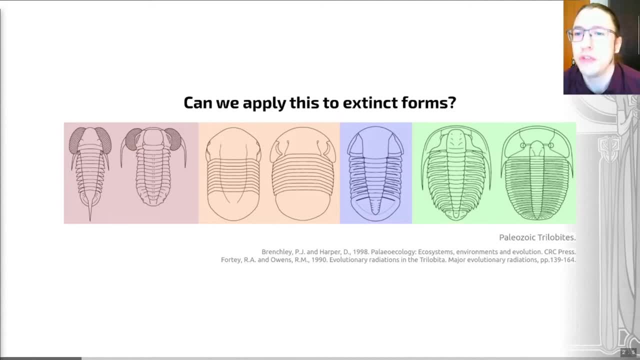 ecosystems And trilobites are super interesting, not only because they're so diverse, but because they show extensive convergent evolution. What we see when we look at the trilobite fossil record, writ large so from a big overview, is that the 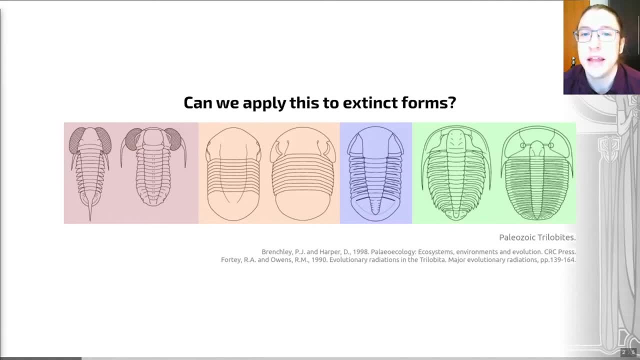 same ecomorphs appear repeatedly in different lineages reflecting convergent evolution to the same life strategies. So an ecomorph is just this idea that you have these morphologies that are tied with the ecologies of these trilobites. 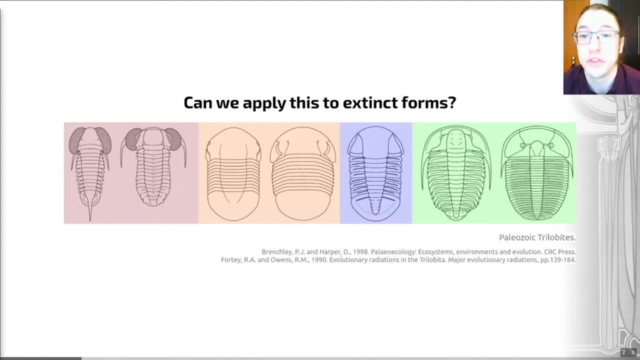 And some examples of that are the trilobites, which is a very similar kind of examples are shown for you on this slide. here In red we have our swimmers. These are creatures that had big, what we would call hypertrophied eyes. They have reduced pleurae. You learnt. 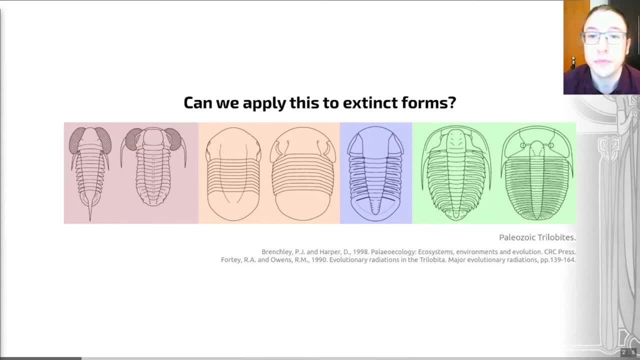 about those when you were doing your characters with Rob, And they appear suited to life in the water column, possibly surface waters. In orange on this slide we have a group called the elanomorphs. These were smooth in terms of their exoskeleton and they were probably 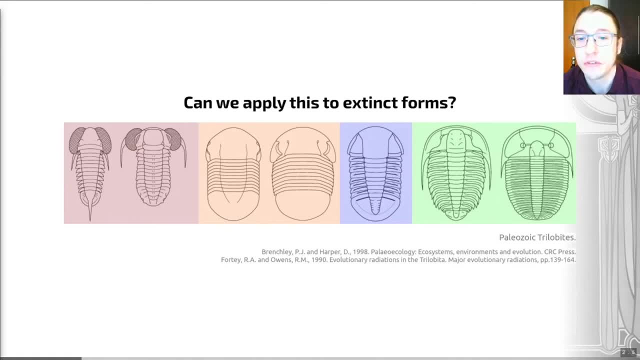 associated with carbonate environments, such as reefs. Their body and their bigidium were probably buried in sediment, with their head resting on the surface. In blue we have the ethyloptic taxa, which have reduced eyes, So eyes were obviously not so useful for them. 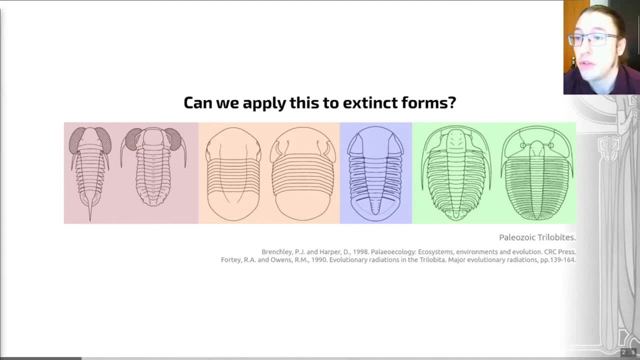 and this means they were probably associated with deep water habitats where there wasn't as much light around. On the far right we have the elanomorphs- These are shown in green- which had a thin exoskeleton. This means that we may associate them with life in diserobic environments. You don't. 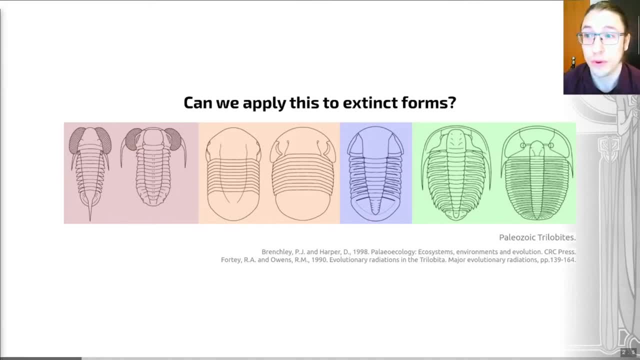 want to be carrying around a heavy exoskeleton that also incorporates oxygen in the form of calcium carbonate into the exoskeleton, And there's not a lot of oxygen around. So this is an example, amongst different groups, of morphological convergence with an adaptive. 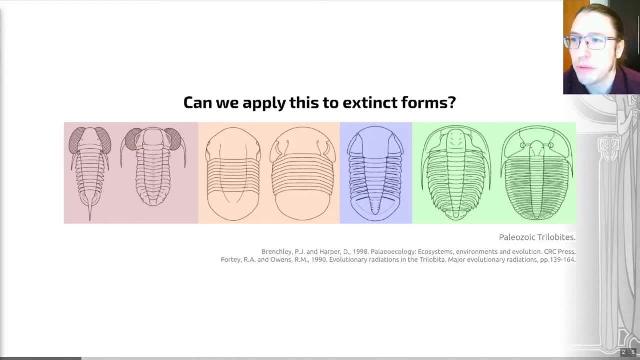 significance And it's very much a thing that you can build up from the first principles. It's not particularly rocket science. We look at these fossil morphologies, we try and understand how they differ from each other and then we draw inferences from that. 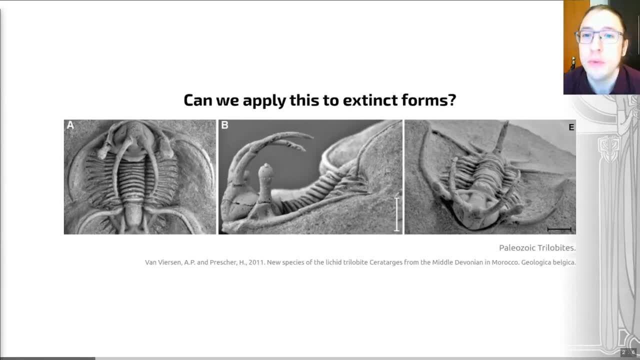 So that's the example of paleo-autoecology. But even with extinct forms, when we can make these sensible deductions, there are limits to what we can say. when we're looking at the fossil record, There are changes that occur within these groups that we can't explain so easily using ecology. An example that I've 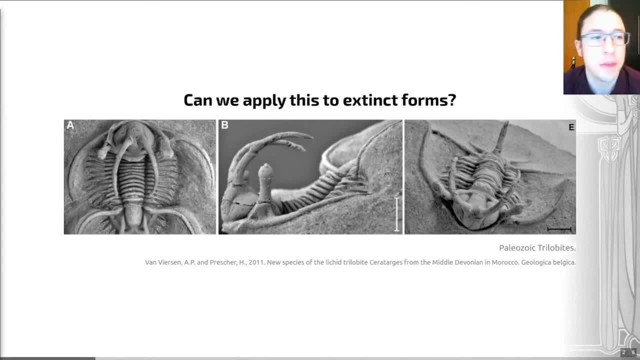 chosen here is the spined trilobites that start appearing in the fossil record in the Devonian. Clearly, there are other selective forces occurring within the group that are not directly related to their ecology. But there are also other selective forces that are occurring within the group that are not directly related to their ecology, And this 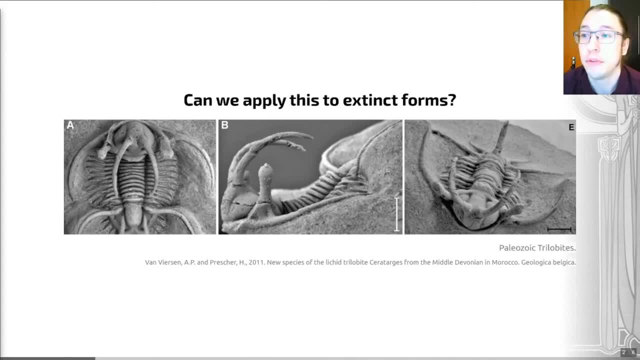 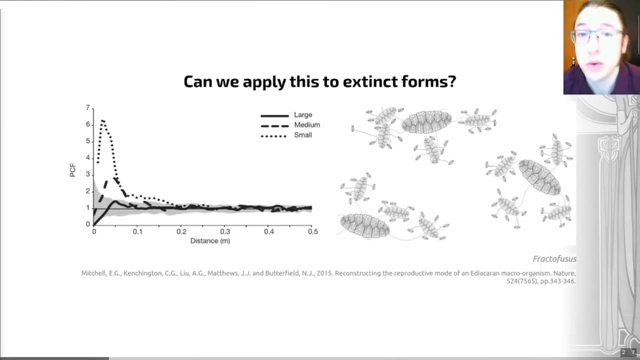 spines may be some form of sexually selected characteristic, but they could also be defensive in their nature, And so we have to take a nuanced approach to trying to understand the paleoecology of fossil species. I wanted to finish with a really cool example of paleo-autoecology, applying this to a completely 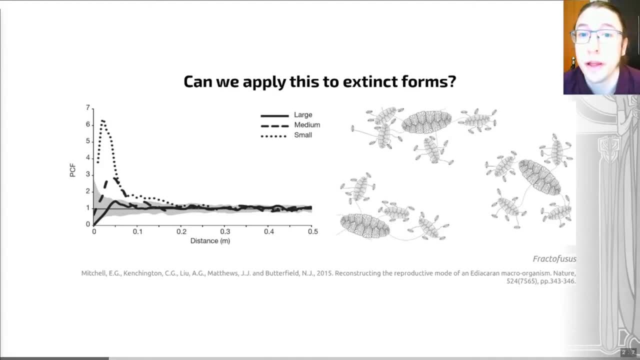 extinct group of animals. So you may remember from lecture number one, the one on evolutionary milestones. So here is the first example of a paleo-autoecology group in our country. The first example of a paleo-autoecology group in our country is a group of creatures that 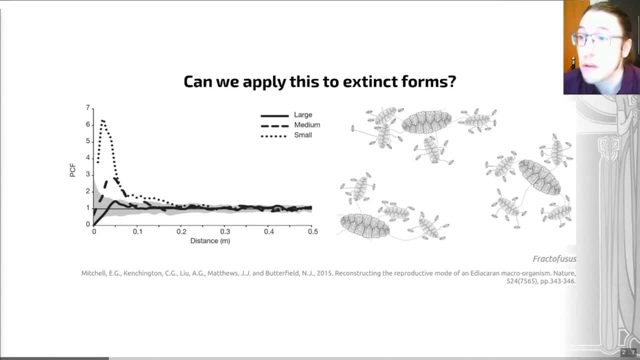 appear at 650 million years ago. They're multicellular organisms. They go extinct before the appearance of major animal phyla, at 542 million years ago or shortly thereafter, And we have absolutely no idea what their mode of life was. In fact, we discussed some possibilities in our first 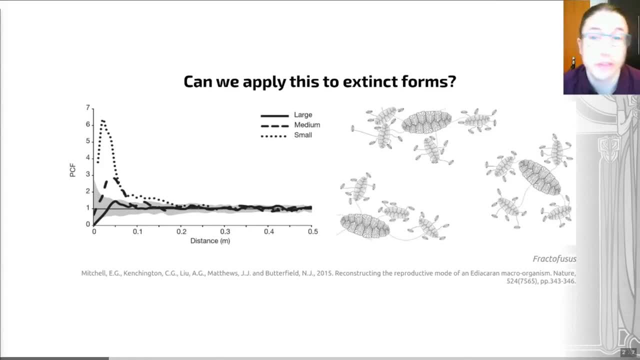 Zoom session, But my example here is based on some work from some very talented colleagues of mine, led by Emily Mitchell, that were published in 2015, and these are using some clever statistical techniques to do to deduce elements of the mode of life of an Ediacan species. So specifically, 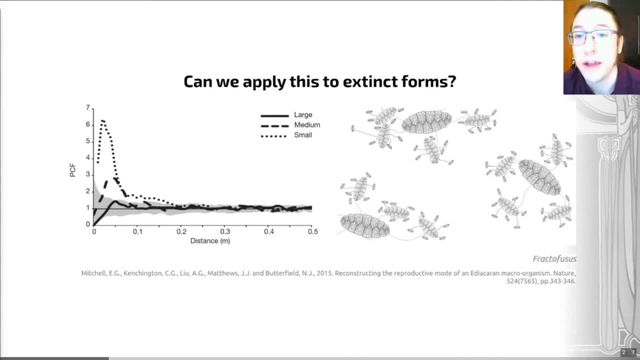 in this paper they looked at how these organisms may have bred. It's really clever, because what they do is they use spatial analysis to investigate the distribution of a single species called Fractifusus on bedding planes. So on bedding planes, so a single surface of rock, you actually 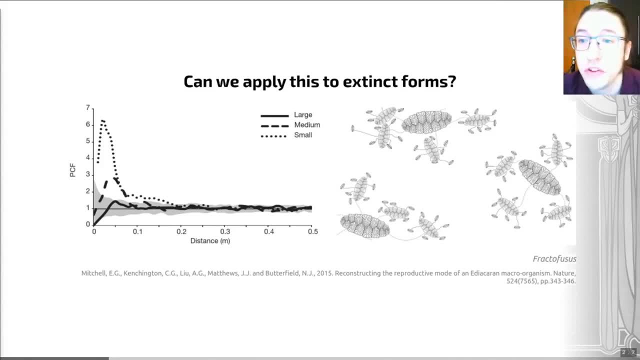 have fossils of a large number of individuals of this species in their life position. This allows you to investigate how they are distributed in space. This graph here shows that. so this is a thing called a pair correlation function, showing the distances between each individual. on this: